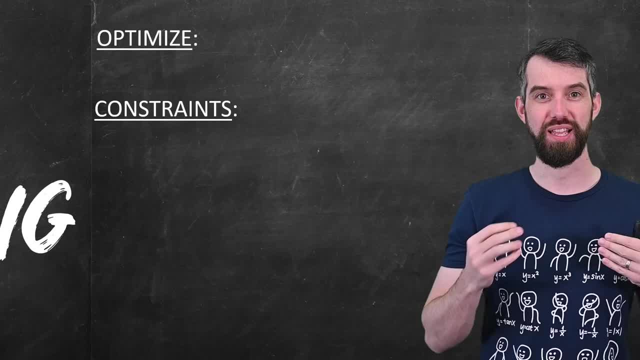 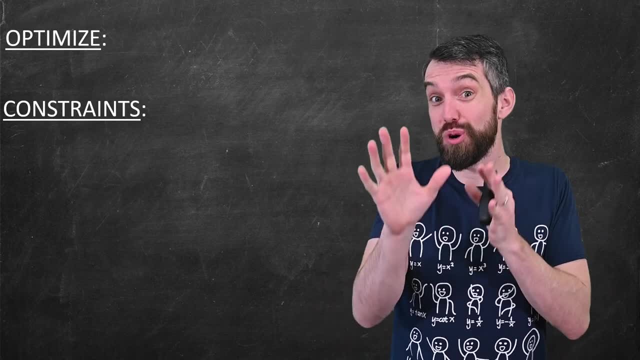 In this video I'm going to tell you about a very powerful optimization technique called linear programming. Now, I know it has the word programming in the name, but we're not actually going to be doing any sort of computer programming here And in fact we're not going. 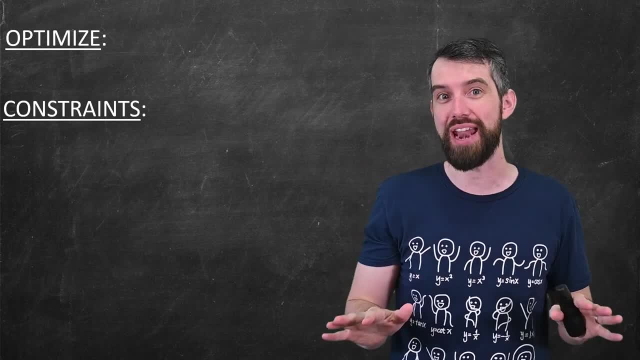 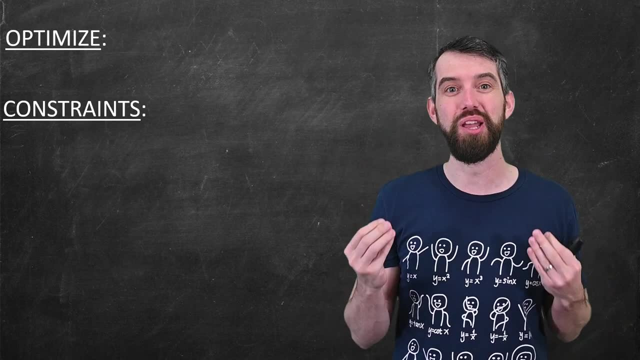 to use any high level math at all: calculus, linear algebra, none of that. Instead, we're going to use a very simple geometric technique that somehow manages to solve this very important class of optimization problems. So what are we talking about? What I'm imagining is I: 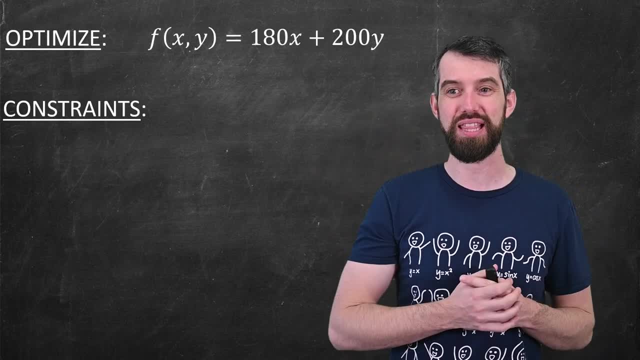 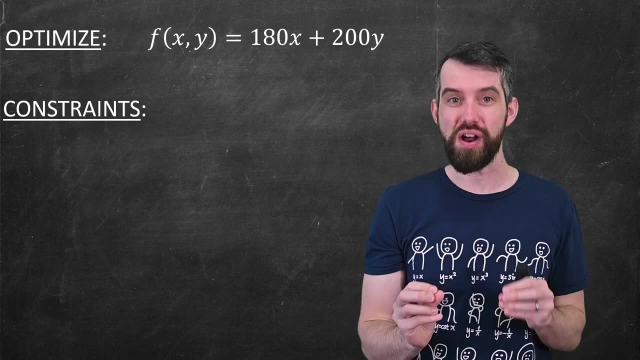 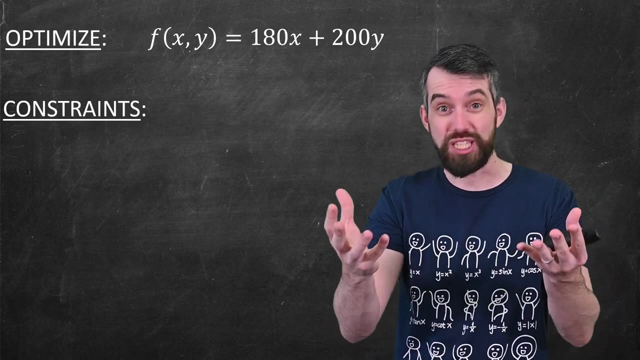 want to optimize the value of some function like this: 180x plus 200y, something like that. That is, this is a linear function of multiple different variables, say x and y. This is just an example. What does optimize mean? Well, it could be find the maximum, or 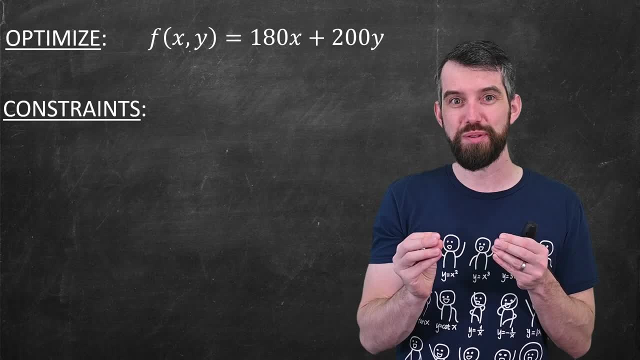 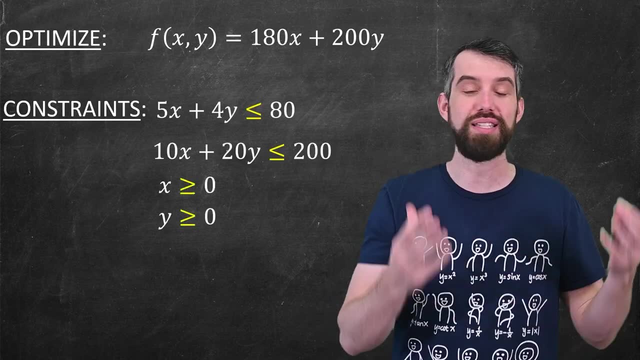 it could be find the minimum. But we're not just optimizing this function by itself. We're optimizing it by itself. We're optimizing it by itself. We're optimizing it by itself. We're optimizing this function subject to various constraints. For example, I'm just 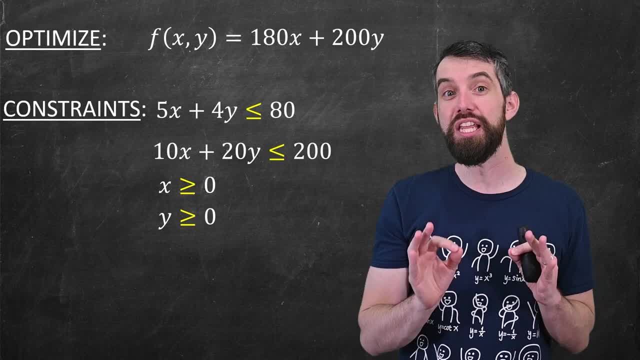 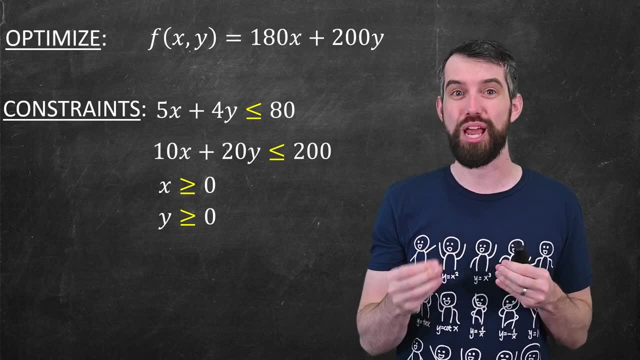 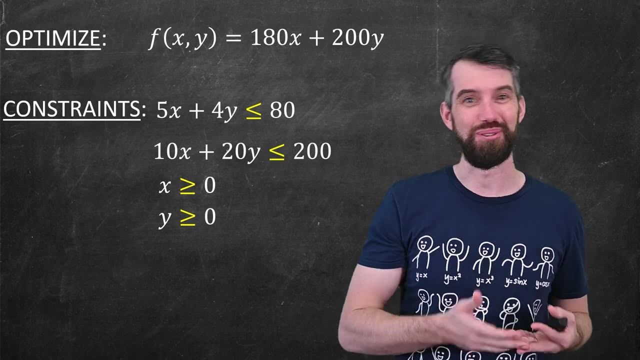 putting up some random ones, a series of what we call linear inequalities, Things like 5x plus 4y is less than or equal to 80, or 10x plus 10y is less than or equal to 200, or x is positive or y is positive. Those are all linear. There's not an x squared or a sign. 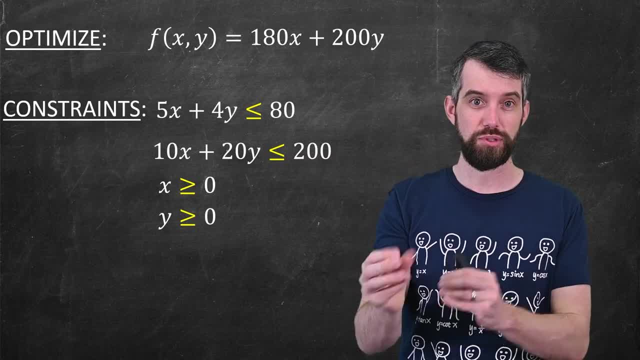 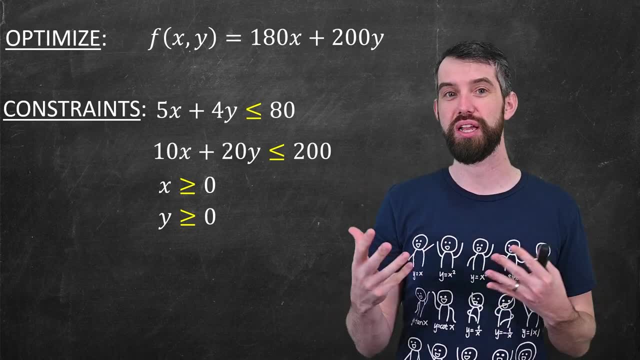 of x, but they're linear inequalities. So this is the idea of linear programming: You're trying to optimize some linear function. You're trying to optimize some linear function. You're trying to optimize some linear function subject to a list of linear constraints, To give an 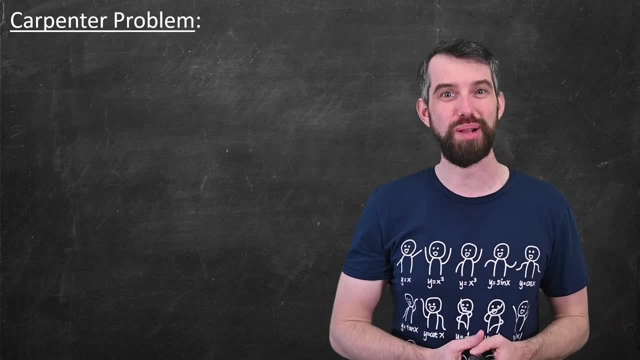 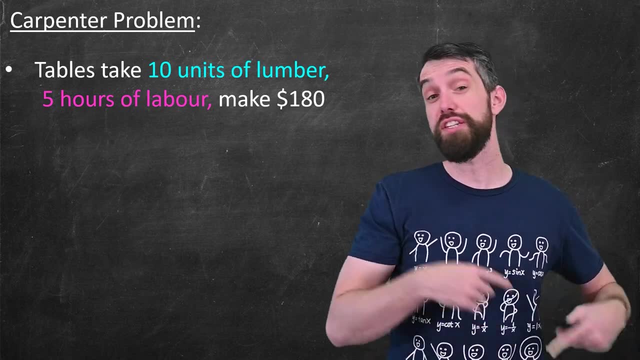 idea of where this type of problem would come up. I'm going to share something called the carpenter problem. The idea is this: A carpenter can make tables, or they can make bookshelves. If they choose. to make tables, it takes 10 units of lumber I don't know anything about. 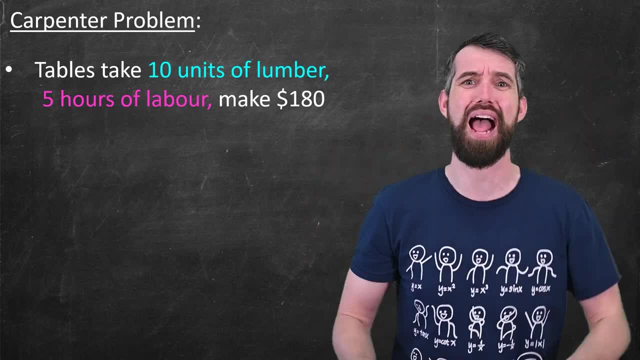 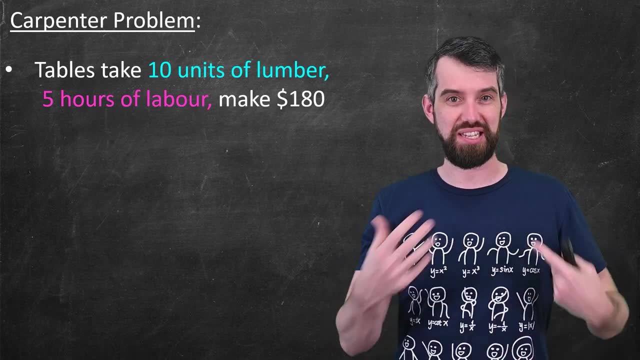 carpentry. I don't know what a unit of lumber is. Some cubic meter? I have no idea. It takes 10 units, however, of lumber, but it takes five hours of work to make a table. So if they make a table, they're going to make 180 bucks profit. Alternatively, if they 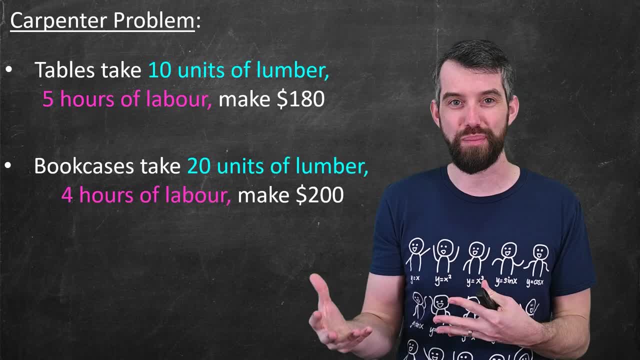 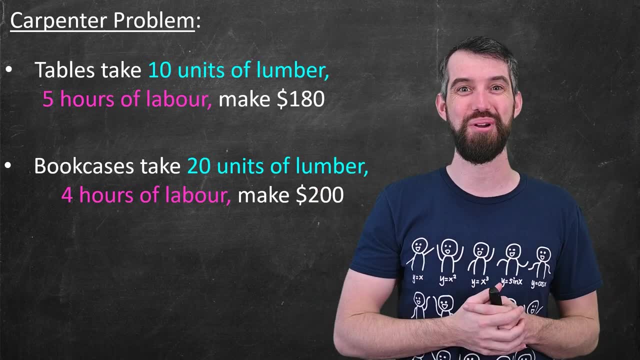 decide to make a bookcase. well, it takes twice the amount of lumber to make a bookcase in this again made up scenario, But it takes less time for whatever carpentry reason. again, I have no idea that claims that bookcases are perhaps easier to put together. So four: 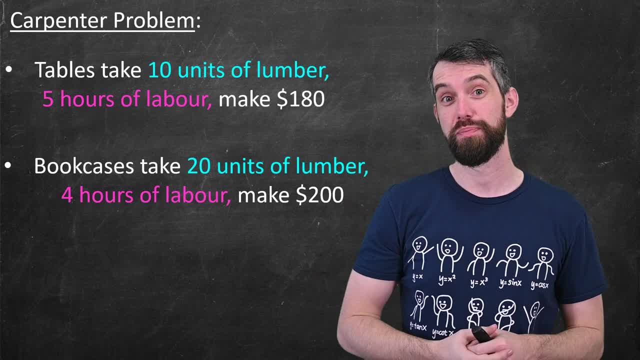 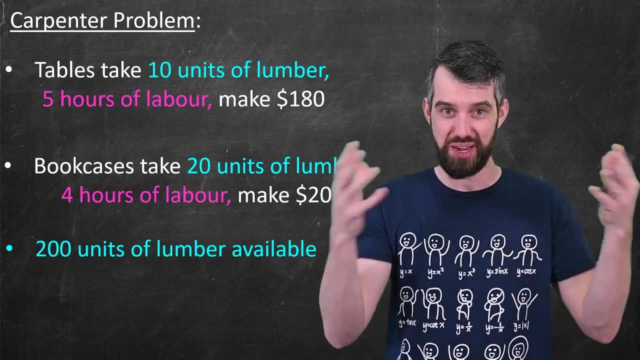 hours of labor, but you make more money- $200.. And then there's a few other constraints here. First of all is that there's only 200 units of lumber available that we can make our bookcases or tables out of. And finally, in say two, 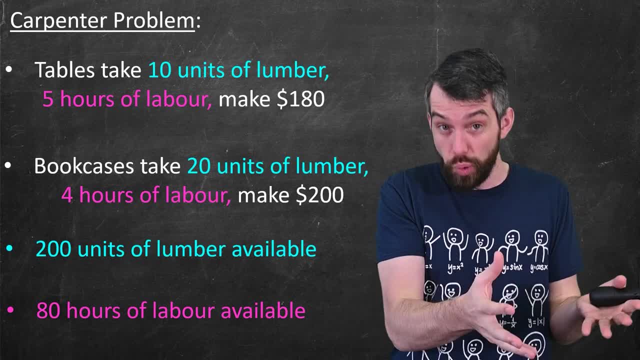 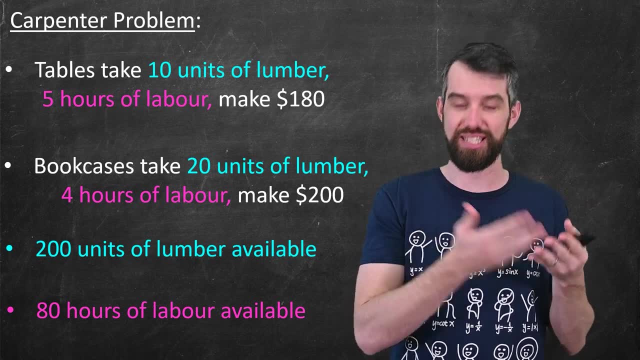 weeks. you want to work only 80 hours. There's a constraint, that is, on the amount of wood, and there's a constraint on the time. Okay, so my first task is going to be to transition this word problem into the system of equations. 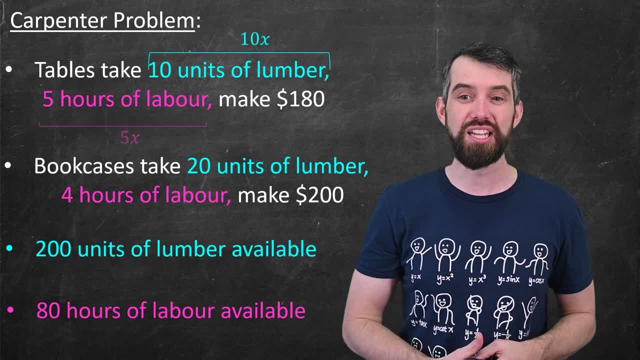 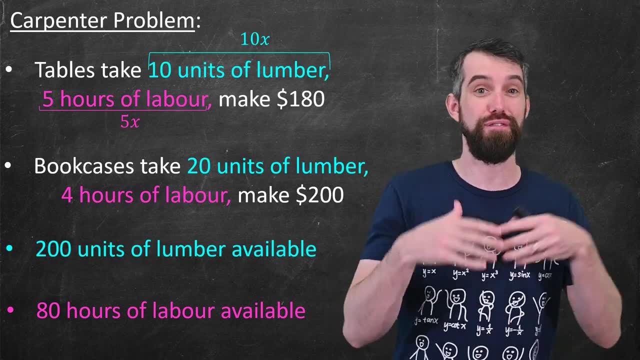 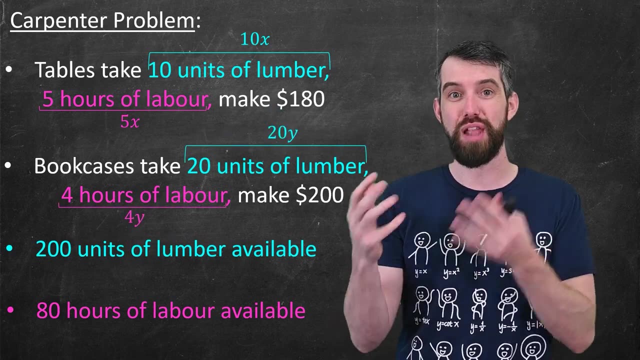 and inequalities like what I just described. So let's let x denote the number of tables, In which case, if you make x tables, you use 10x units of lumber and 5x hours of lumber. Likewise, I'll use y to denote my number of bookcases, And so 20y is the amount of. 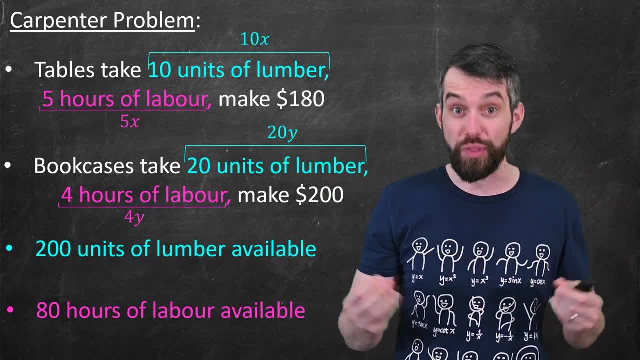 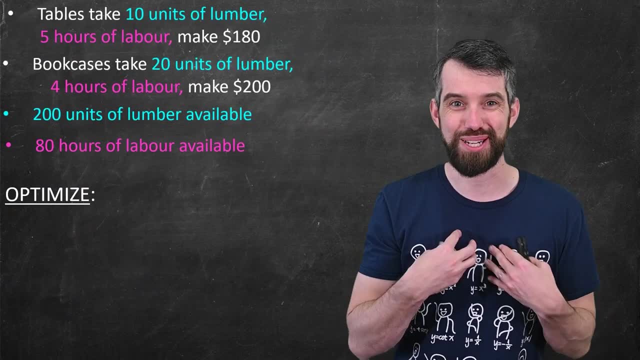 lumber I use and 4y is the amount of labor that I use. So if I condense these equations down, then the question first of all is: well, what am I trying to optimize? Well, I want to make as much money as possible. That's the goal. 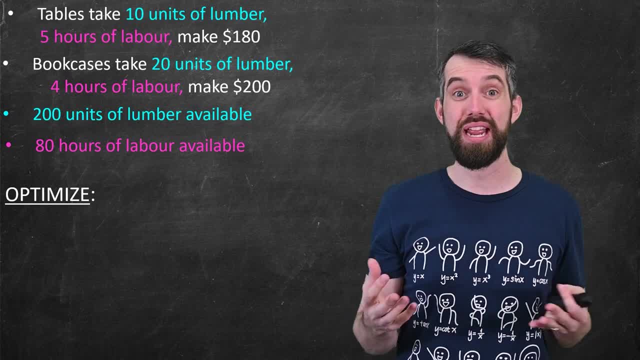 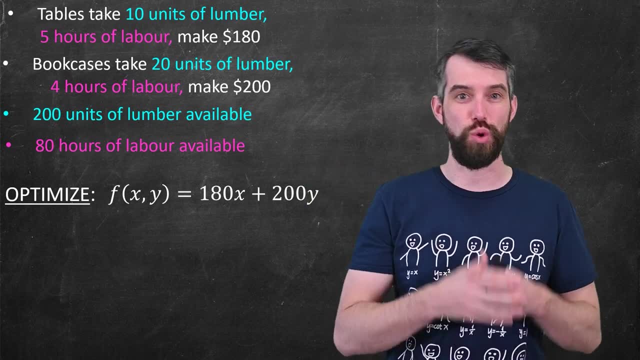 here, right? So what's my money going to be? Well, I make $180 for every table that I make and $200 for every bookshelf that I make. So the thing I want to optimize is this function, this linear function: 180x plus 20x. 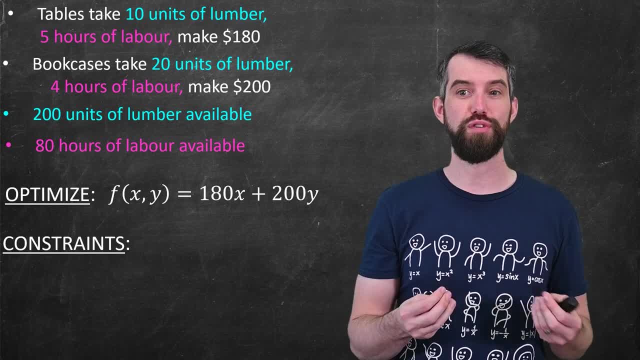 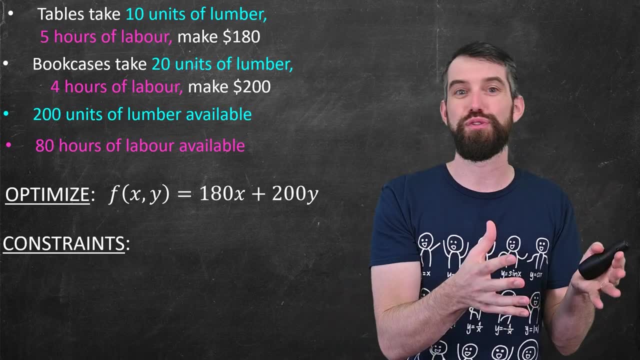 What are y? Okay, so what about my constraints? Well, first of all, let's think about the constraints on my labor, the number of hours that I can spend on this. So the rule is five hours for a table, four hours for a bookcase And, as a result, 5x plus 4y has to be smaller. 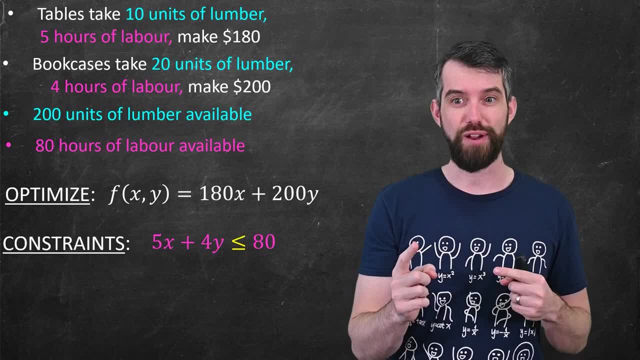 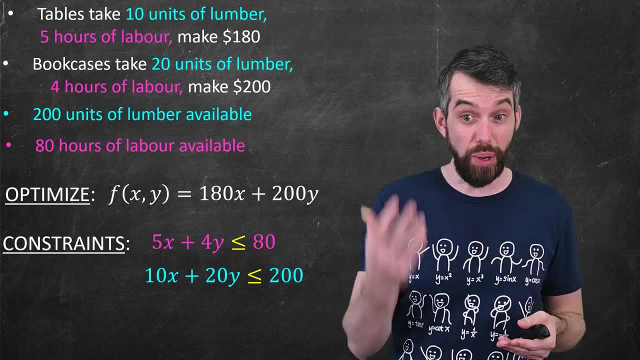 than the 80 hours that I'm willing to work. Then, if I want to consider the constraints on the lumber, well then 10 times the number of tables plus 20 times the number of bookcases has to be less than the 200 units of lumber. 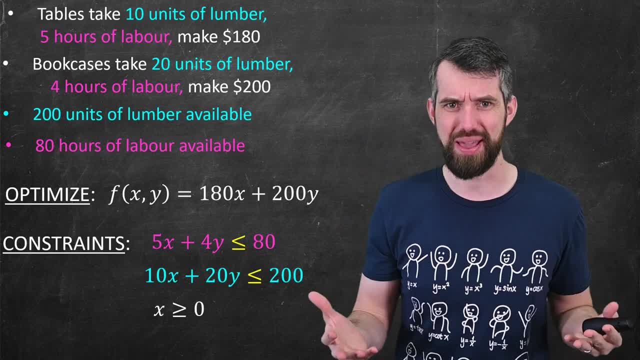 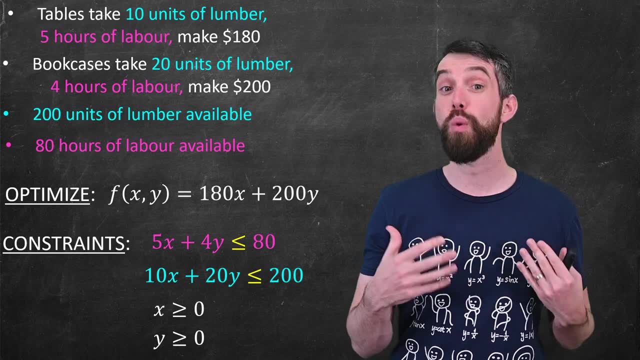 that I have, Again, another inequality. Finally, the number of tables I make is going to be a positive number, And likewise for the number of bookshelves, I'm not going to make a negative number of tables. Okay, so now I want a procedure to be able to solve these, And I'm going to introduce 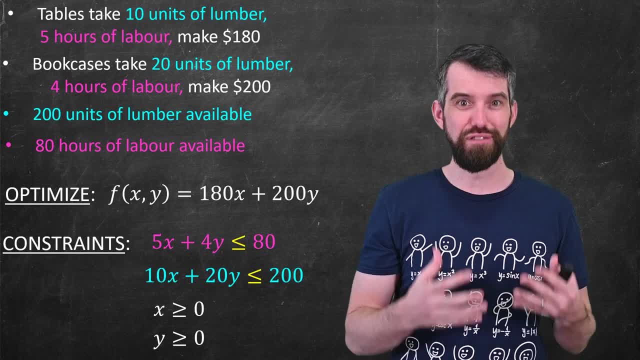 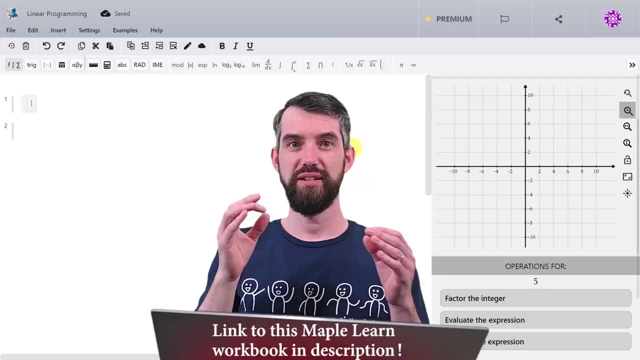 something called the simplex method. Before I do that, I just want to visually understand what are these inequalities actually saying, And for that we turn to the computer. To help me graph these inequalities, I'm going to turn to Maple Learn, which is actually. 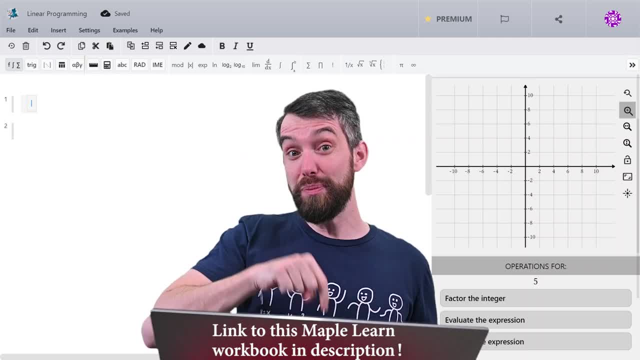 the sponsor of today's video. Maple Learn is a software that allows you to graph the number of tables that you make. Maple Learn is a software that allows you to graph the number of tables that you make. If you go down in the description, you can check out for free either the web application. 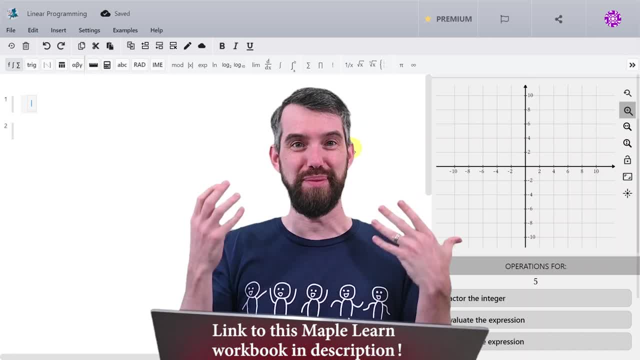 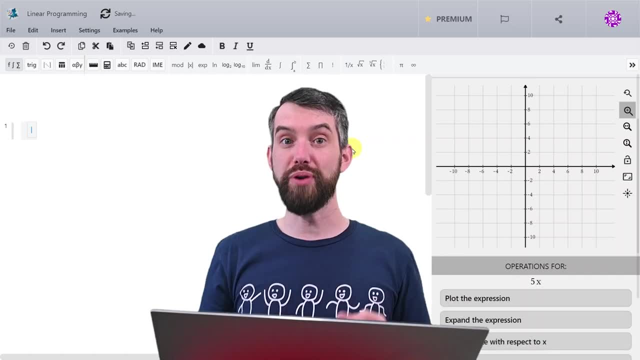 Maple Learn, or the phone-based app which is the Maple Calculator. Both of them are pretty cool and allow you to do the following thing, which is to graph an inequality. So what are we trying to study? Well, we have the first inequality, 5x plus 4y, and that 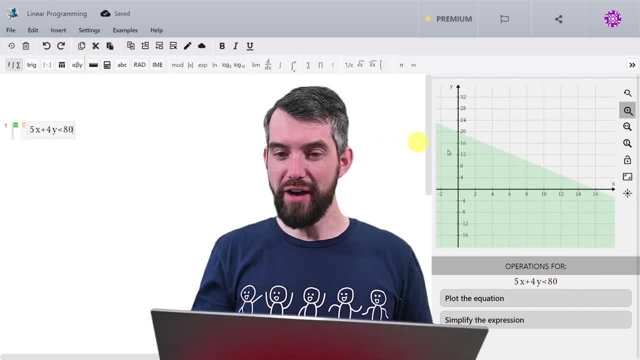 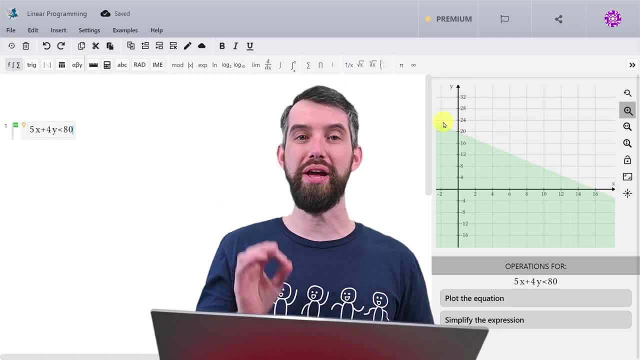 was supposed to be less than 80. And what we have on the right-hand side is a plot of this inequality, And the idea is that along this line- This is the equation- 5x plus 4y is equal to 80. So the fact that I'm asking less than 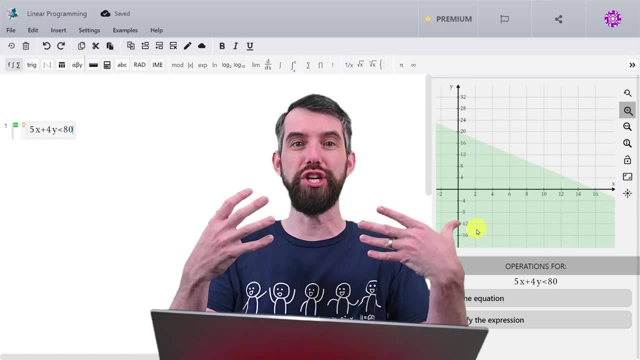 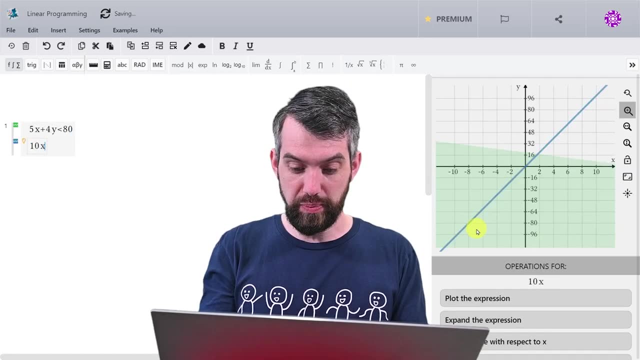 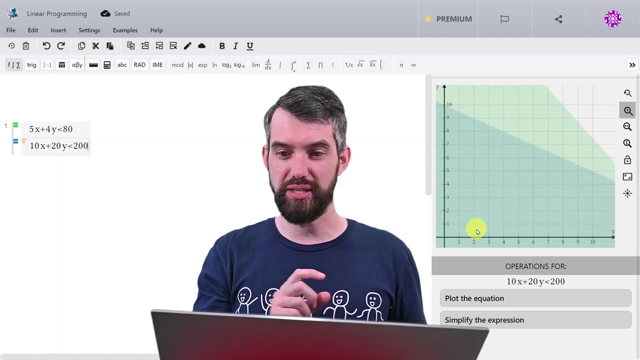